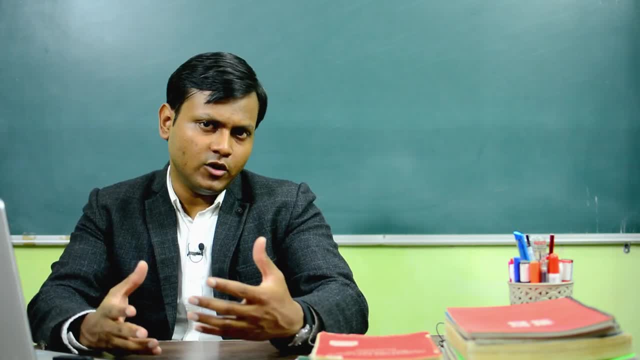 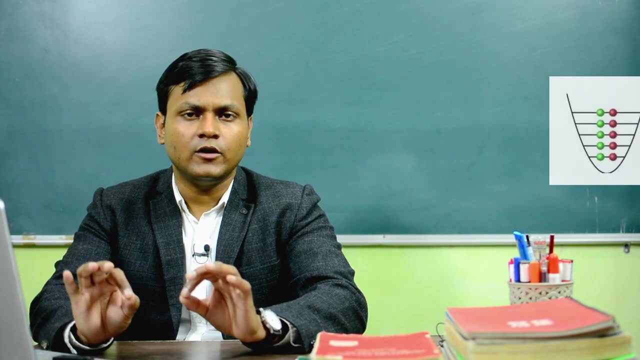 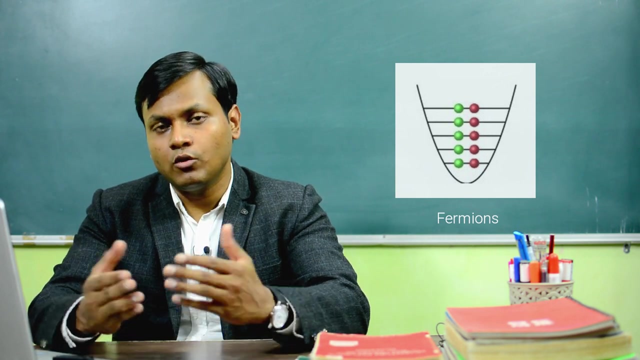 which simply states that if there is a collection of fermion particles and there are energy levels in that kind of a collection of fermion particles, then no more than two of the fermion particles can occupy the same energy level, and even in that case they will have different spin or opposite. 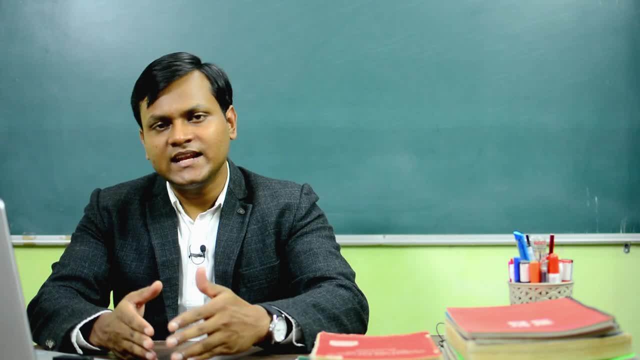 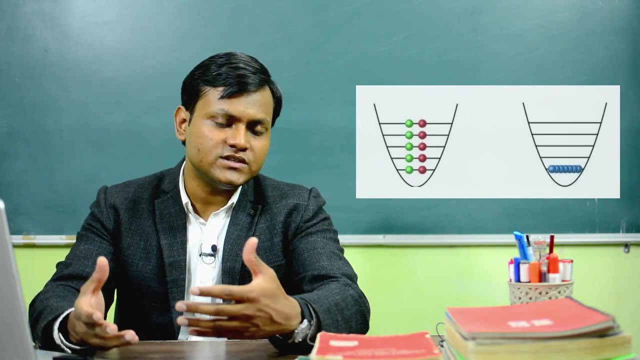 spin. Now, unlike fermions, there are also fermions which are not fermions. So there are fermions. there is another class of quantum particles, known as boson particles, which do not follow the Pauli's exclusion principle. So in the case of bosons, if there is a collection of boson particles, 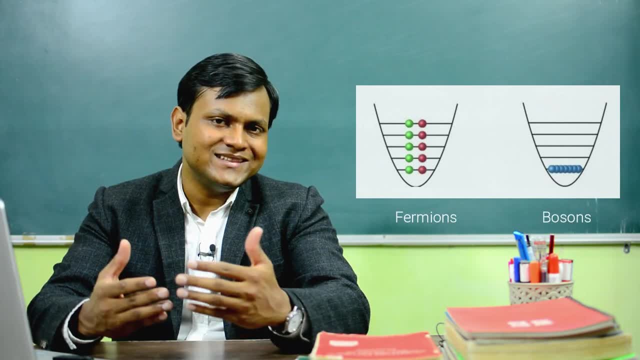 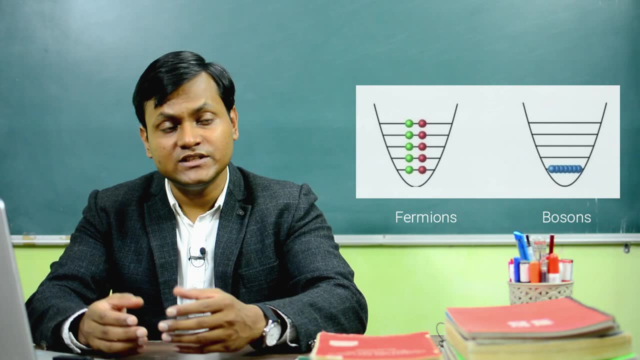 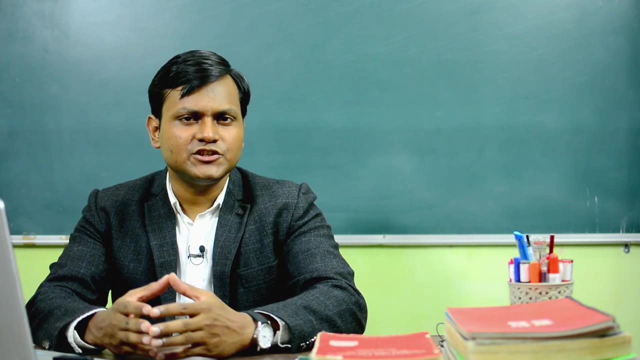 then n number of boson particles can occupy the same energy state. So, unlike bosons in the case of fermions only two of these particles can occupy the same energy state. That means only two particles among a collection of particles can share the same energy values. Such a collection 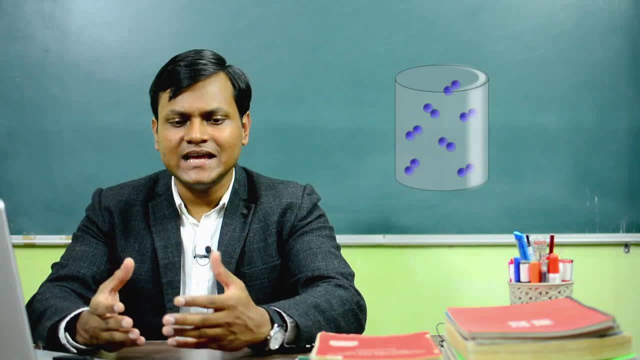 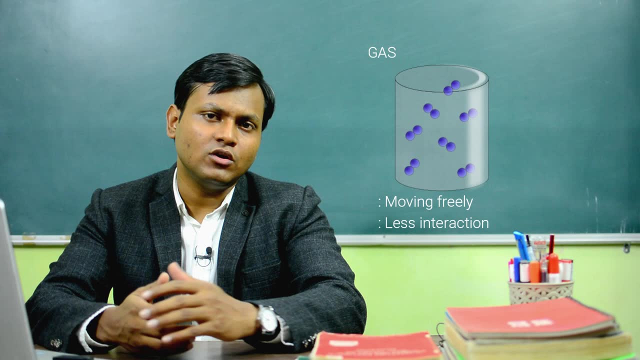 of particles is known as fermion gas. Now what is meant by gas here? Gas simply means that the collection of particles are not interacting with each other, So gaseous state is usually distinguished from liquid and solid state in the sense that in gaseous state most particles or 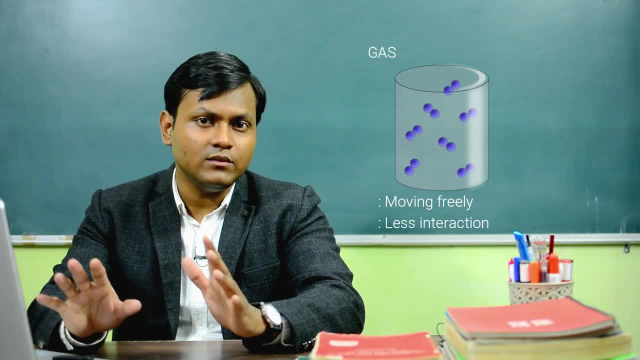 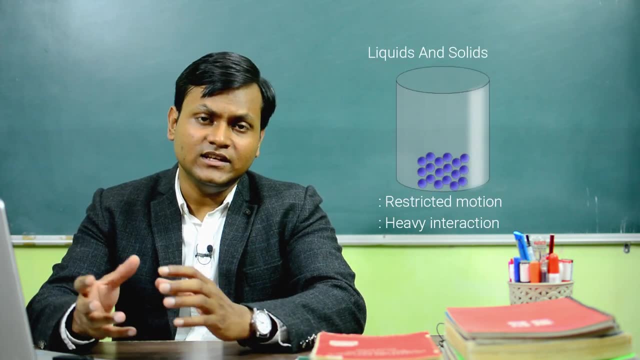 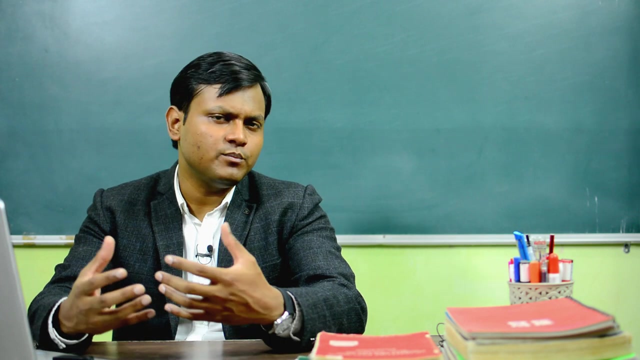 individual molecules are moving freely most of the time and they are only interacting with the nearest neighbors very rarely, as opposed to liquids and solids, where the particles are interacting with its nearest neighbors almost all the time. So fermi gas is simply a form of a collection of such fermion particles which are moving freely in a given volume. Now how can such 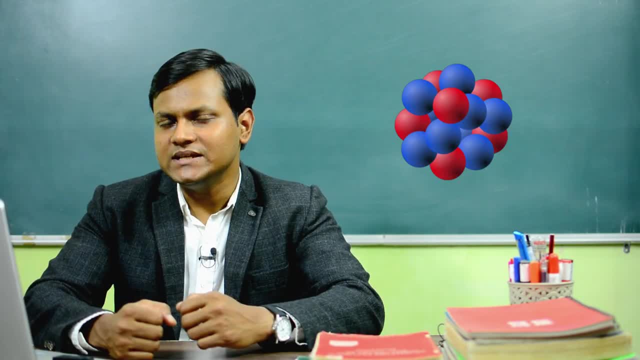 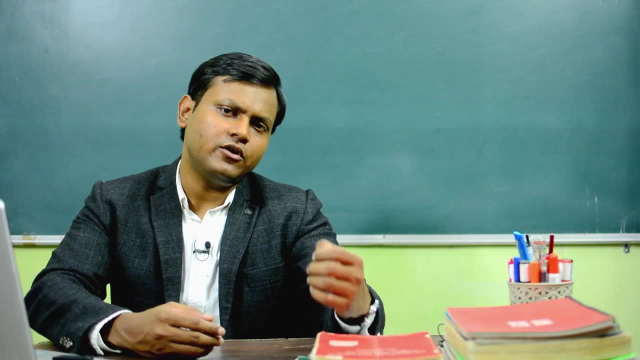 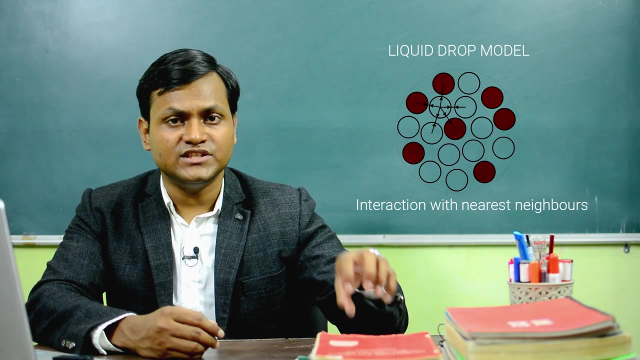 a fermi gas model be used to replicate a nuclear model. A nucleus is a very small, dense, compact quantum object and if you have seen my earlier video on the liquid drop model of the nucleus, there I made an assumption that each particle inside the nucleus is interacting only with its 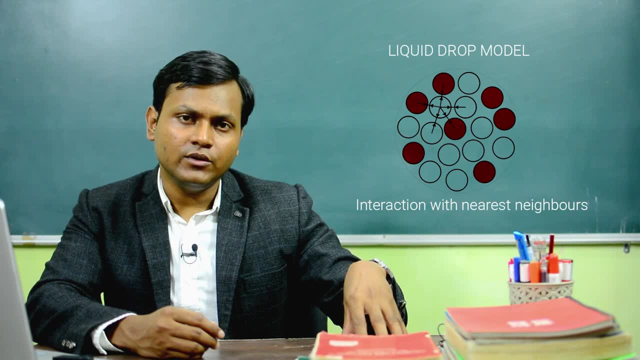 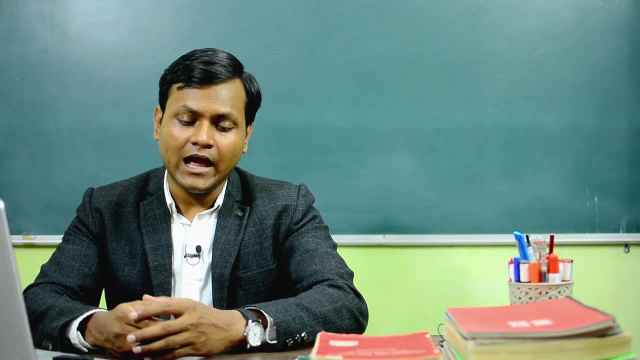 nearest neighbors. So in a sense, the assumptions of the liquid drop model are very different from the assumptions of fermi gas. So in a sense, the assumptions of the liquid drop model are very different from the assumptions of fermi gas. In the assumption of the fermi gas model we assume 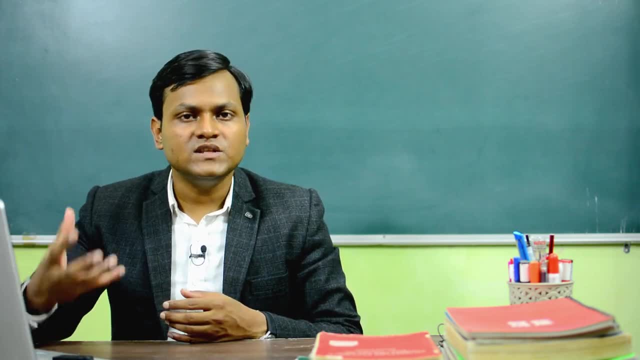 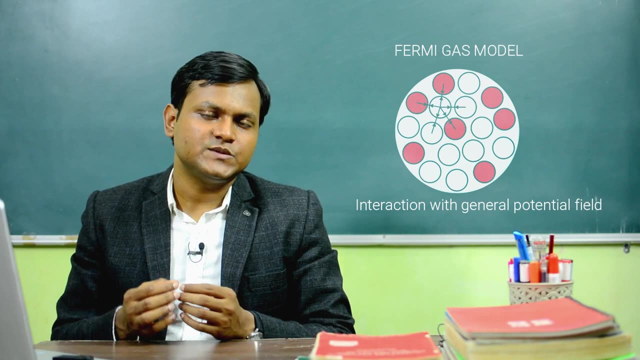 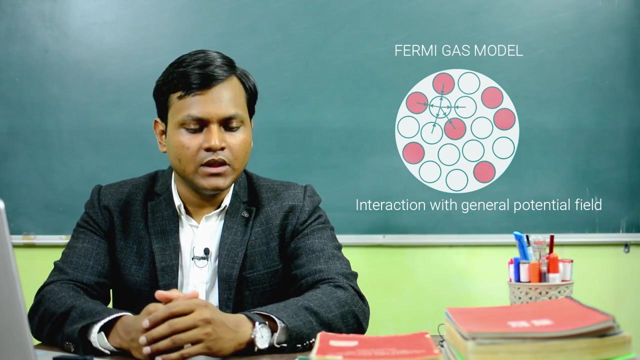 that the net effect of the interactions of each particle with its nearest neighbors can be approximated to be a result of an interaction with a general potential field. So each particle is present in some general potential field and each particle is independently interacting with the general potential field. Now, inside a nuclear volume, the mass density of the particles is almost 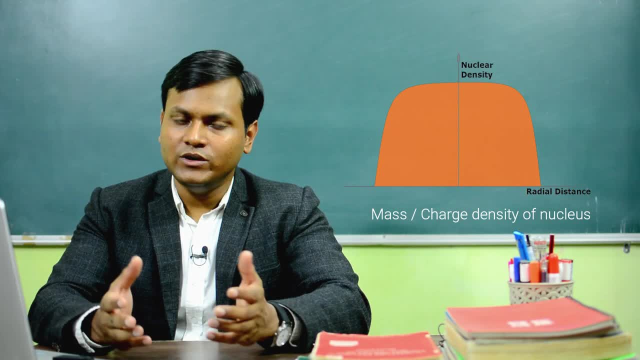 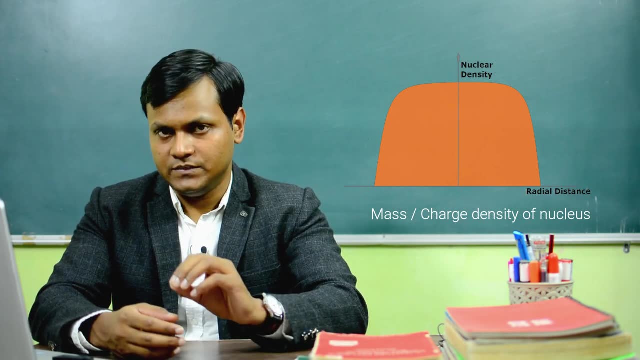 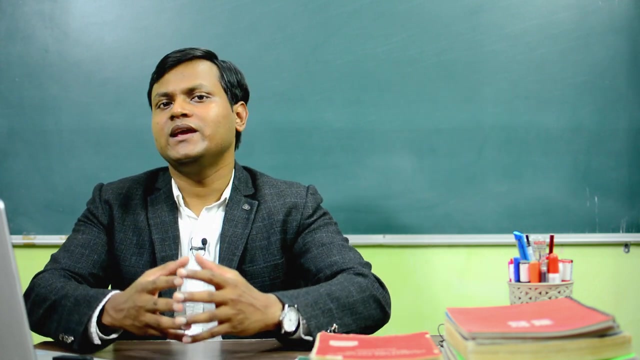 constant throughout the nuclear volume and it drops to zero only near the boundary. So it can be assumed that whatever potential exists inside the nucleus has a constant depth for the entire volume of the nucleus and it drops to zero sharply near its boundary. So basically we can approximate. 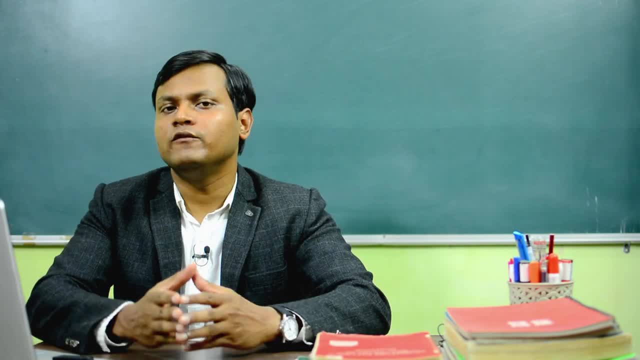 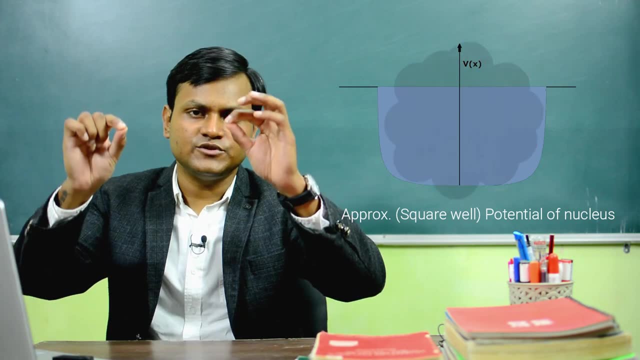 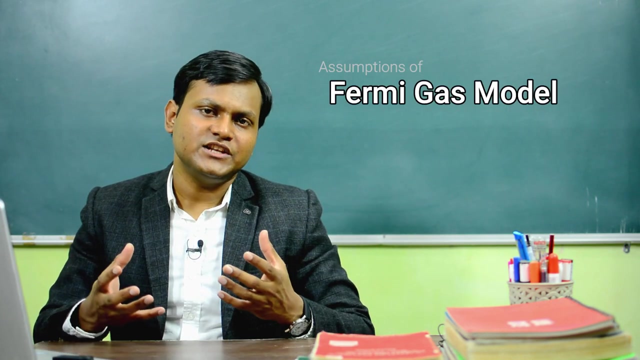 the general potential field of the nucleus with that of a square well potential. So a square well potential has constant depth for a particular distance and it suddenly drops to zero near the boundary. So in the Fermi gas model of the nucleus, therefore, the nuclear potential is approximated by 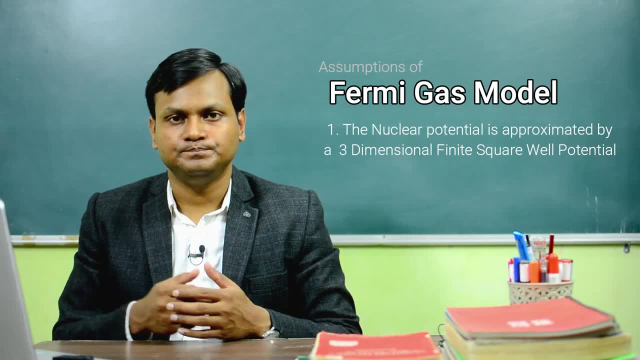 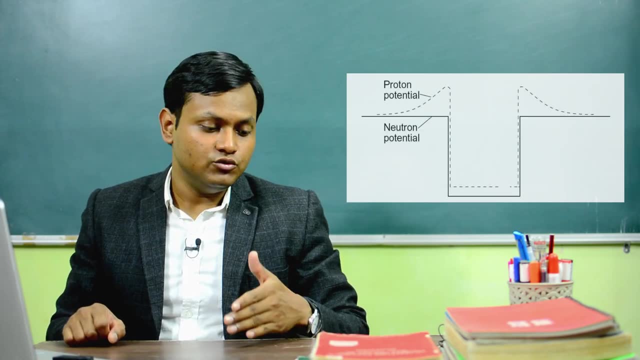 a three-dimensional finite square well potential. Since neutrons and protons are fundamentally distinct particles, their potential wells are also going to be distinct. Neutrons interact with each other via the nuclear force. protons interact with each other via the nuclear force, as well as the. 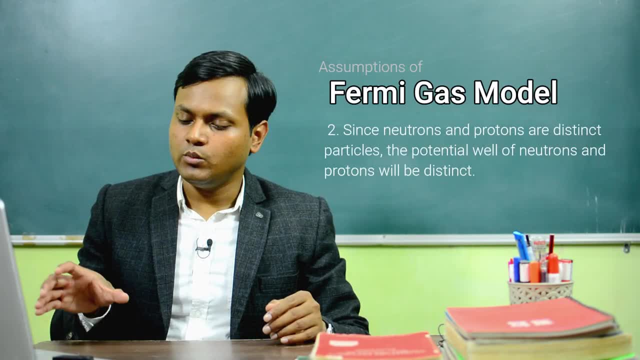 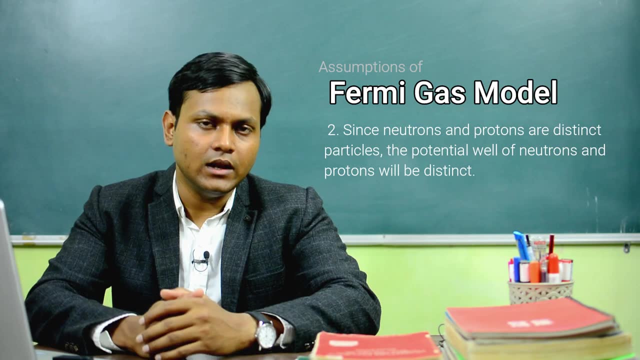 coulombic repulsion. So the potential well of neutrons and the potential well of protons will be distinct from each other and the neutrons and protons will occupy energy levels in their own potential well, Since neutrons and protons are fermions, so no more than two of these neutrons 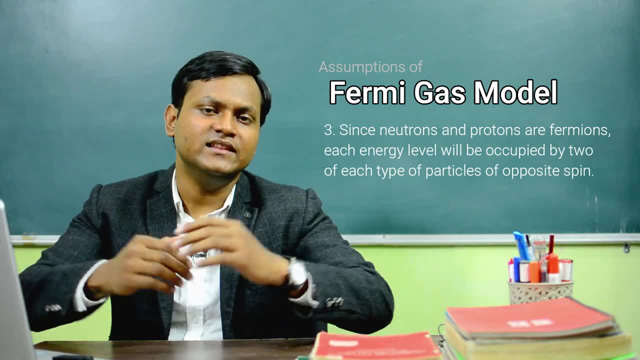 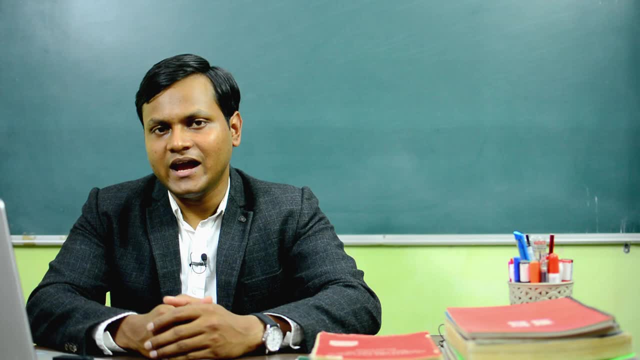 and protons can occupy one given energy level in their own individual potential. well, energy diagram. Now, in the ground state configuration of such kind of a nuclear well structure, almost all these particles will be distinct from each other, So the nuclear force will be distinct from each other. 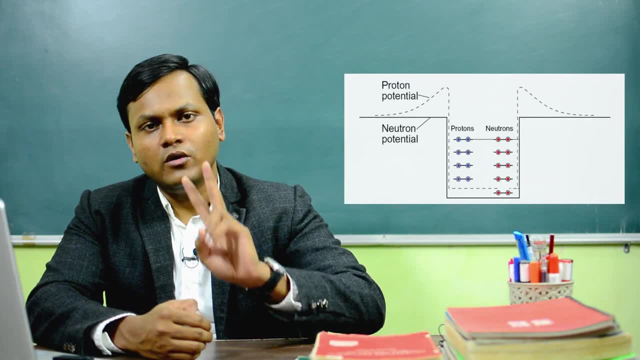 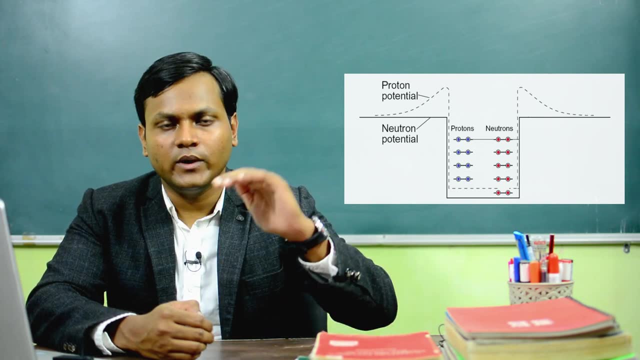 and the neutrons will try to occupy the minimum energy level. So two of the particles will occupy the ground state, the another two particles will occupy the first excited state, another two particles will occupy the second excited state, and on and on and on. So the minimum energy configuration. 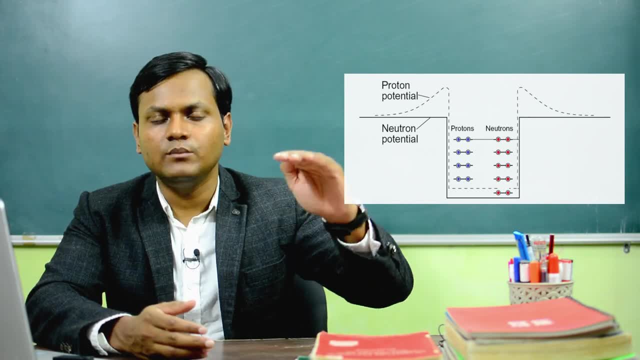 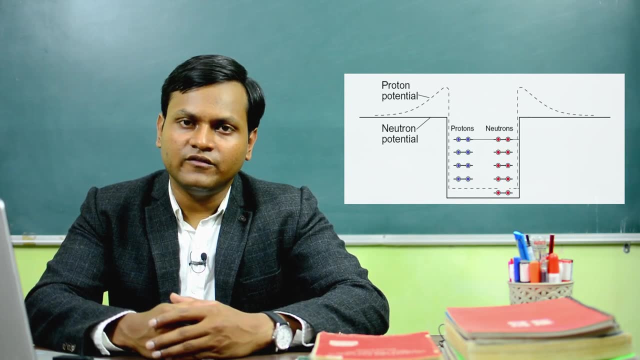 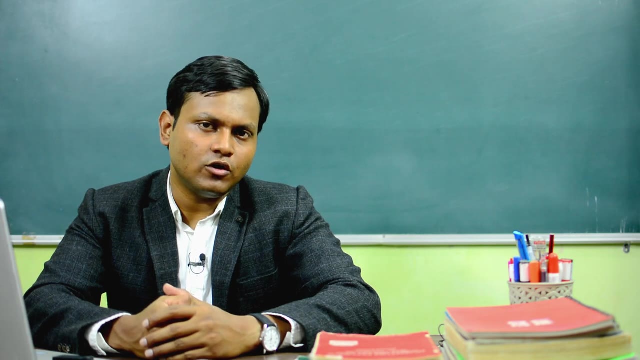 will consist of a large number of particles which fill up these energy levels, one at a time. So, even at zero temperature, even at ground state configuration, the combination of the energies of all of these non-zero, In such a ground state configuration where all the particles occupy the minimum energy. 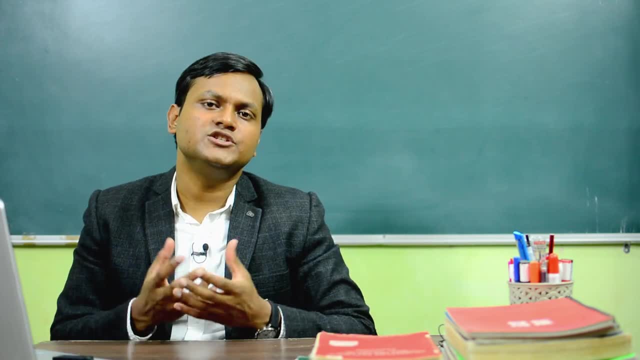 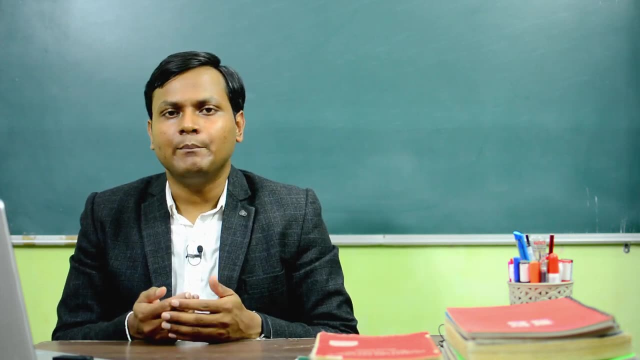 levels possible, then the nucleus can simply be assumed to be a collection of particles where each particle has certain energy which is different from each other. Now what is going to happen if two neutrons come together and collide with each other? Let's suppose there are two neutrons which are at 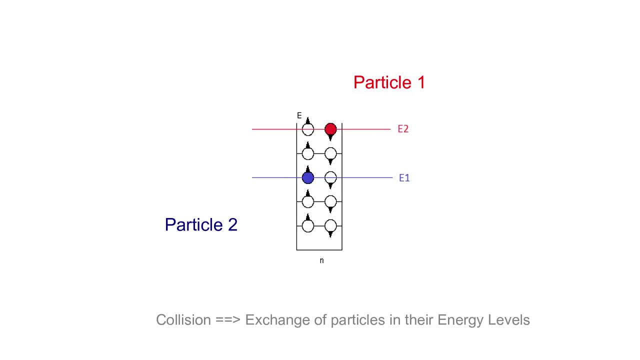 two distinct energy levels and they are moving inside the nucleus and if they come and collide with each other, they simply will not be able to collide with each other, So the neutrons will be will result in the exchange of their energy levels. That's it, Classically. if two particles come and 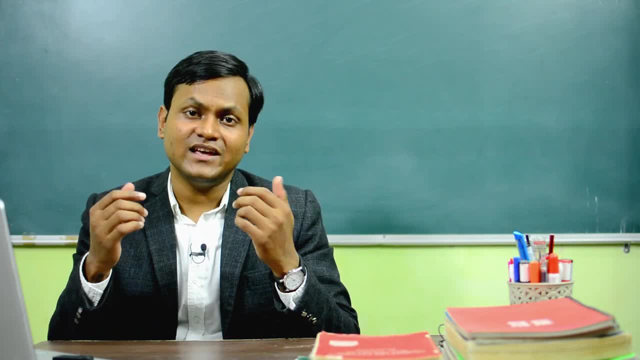 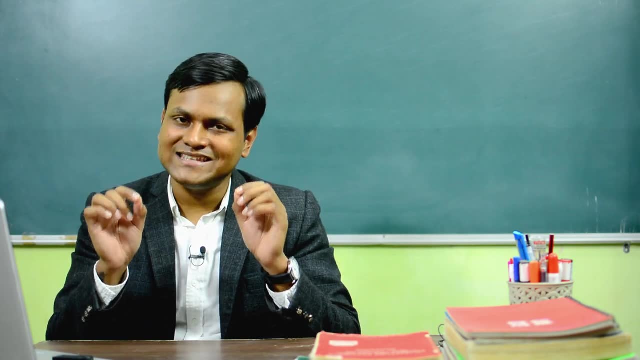 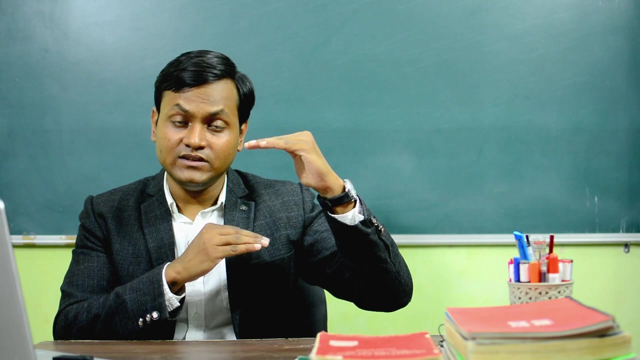 collide together, then in an elastic collision they basically exchange their velocities, right? But in the case of quantum particles, since these two particles cannot occupy the same energy level- and let's suppose these two particles are basically moving inside the nucleus and they occupy different energy levels in the energy level configuration- then a collision would. 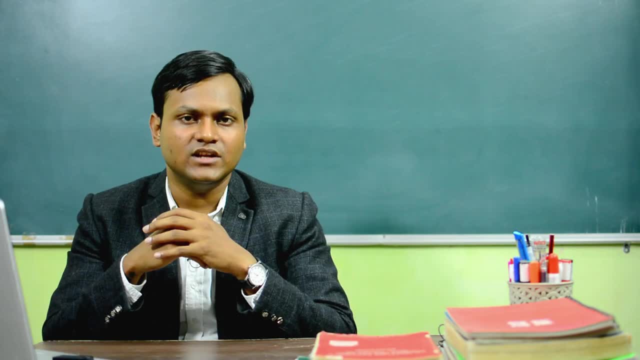 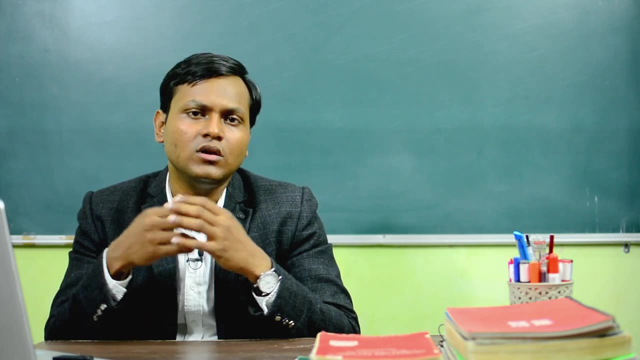 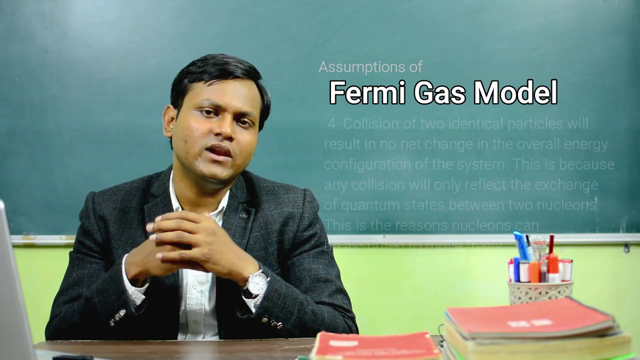 simply represent exchange of these two particles in their energy levels. Now, since these two particles are identical in nature, there will be no difference in the overall configuration of the entire system. So, basically, a collision will lead to no net change in the overall energy configuration of the system. So therefore, we can assume that this collection of 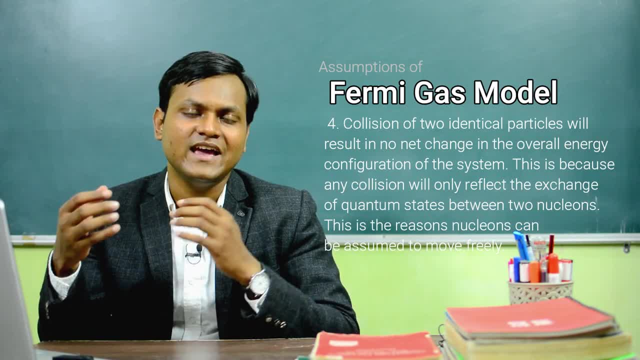 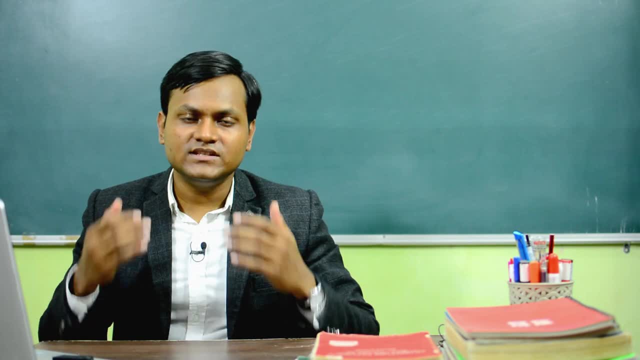 particles, which consists of a lot of neutrons and lot of protons, having different energies, are moving independently of each other, not interacting with each other. So this is the reason we can assume that these two particles are identical in nature. Now, since these two particles are, 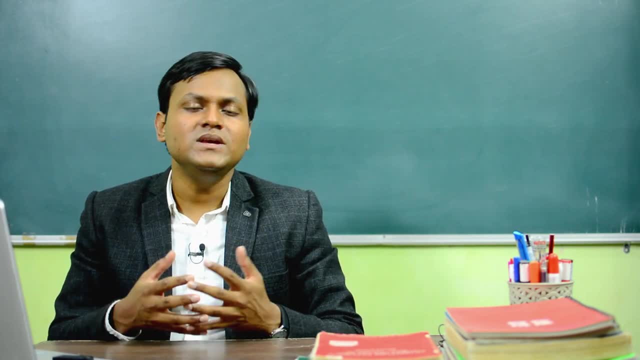 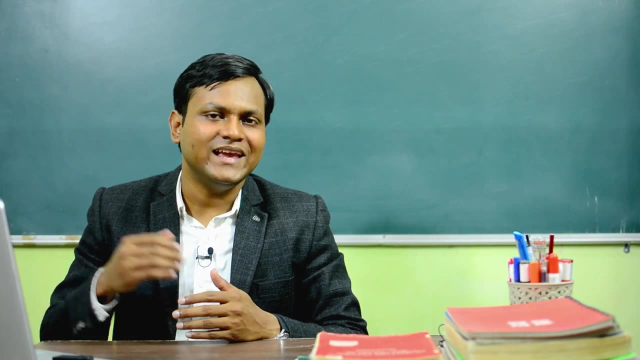 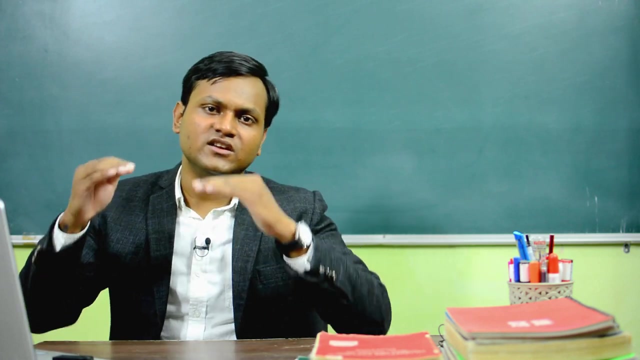 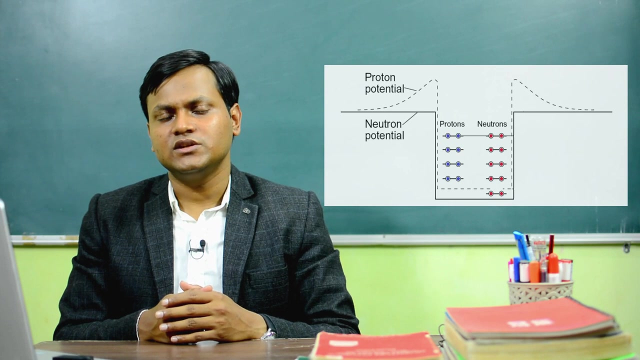 actually interlinked with one another. I know that something of almost any particle will be similar species to any other existing particle of any smallerned nature, And so it's conventionally sufficient for a reaction, because there is nothing allowable Now in the ground state configuration. the highest occupied state has a certain energy. 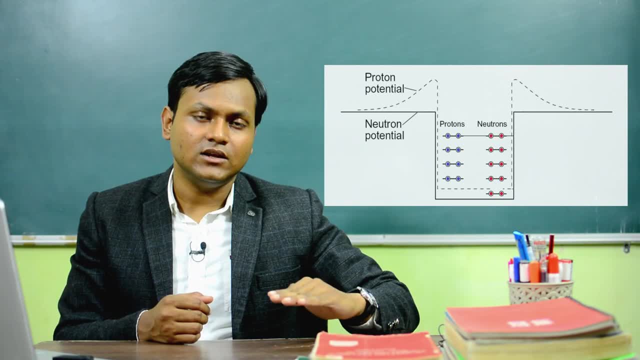 and this energy minus the lowest occupied state meets the lowest occupied state and in the field state, while the above was different. So this is the type of energy that will happen in both planets state is known as the Fermi energy of the given system. Now there is a way to. 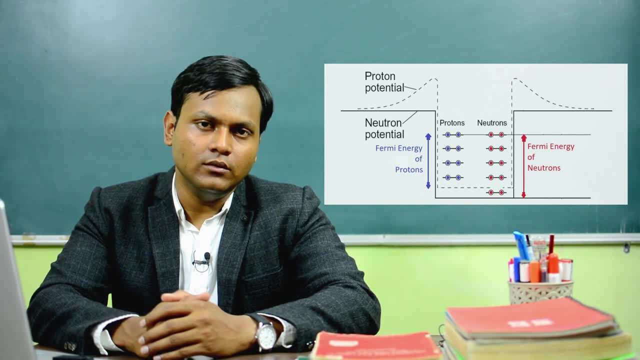 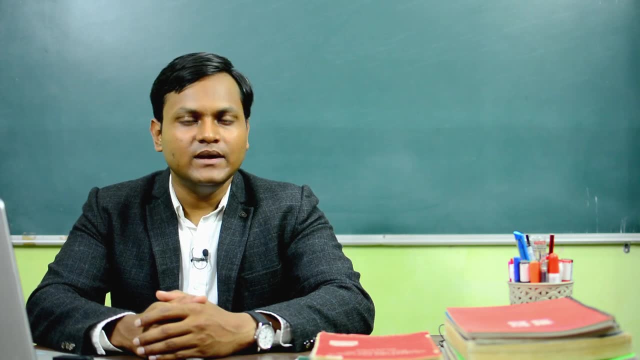 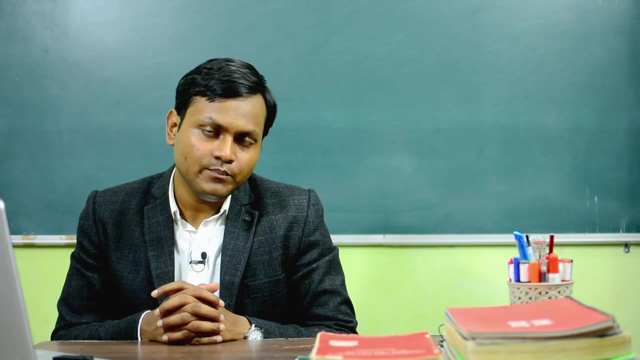 calculate the Fermi energy of a nuclear model. In my previous video I calculated the Fermi energy of both neutrons and protons for a typical nucleus. I basically assumed that the nuclear structure resembles a three-dimensional finite square, well potential and by using the expressions for the quantum. 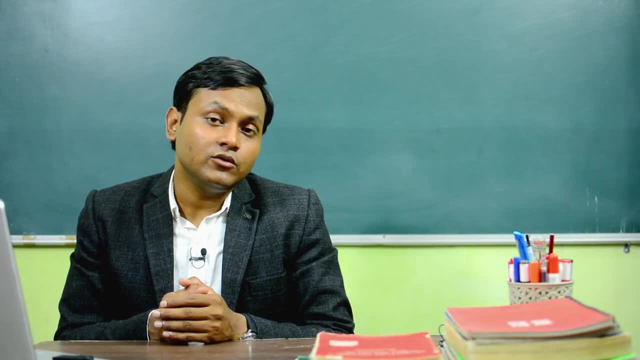 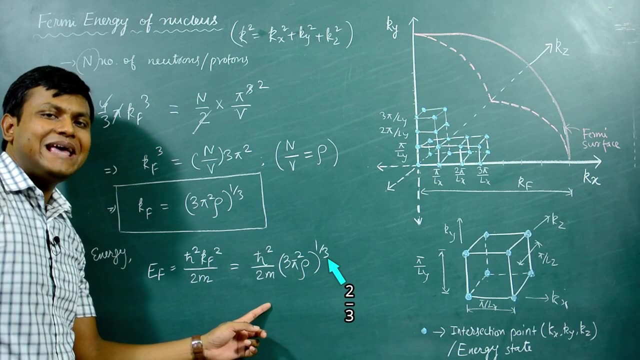 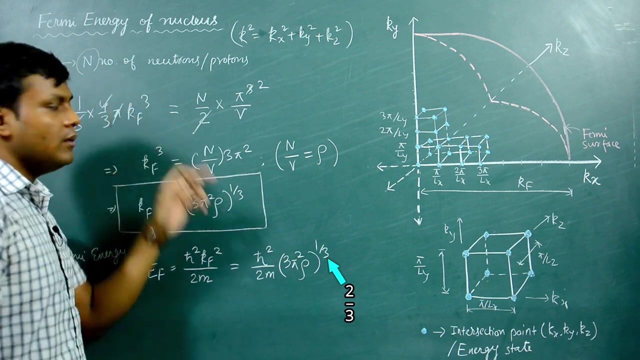 mechanical solutions of the energy diagram. I calculated the Fermi energy for both a nuclear potential well and a proton potential well. This is the Fermi energy, or approximately the Fermi energy of a square well potential which contains n number of neutrons, and according to my calculations, I found out: 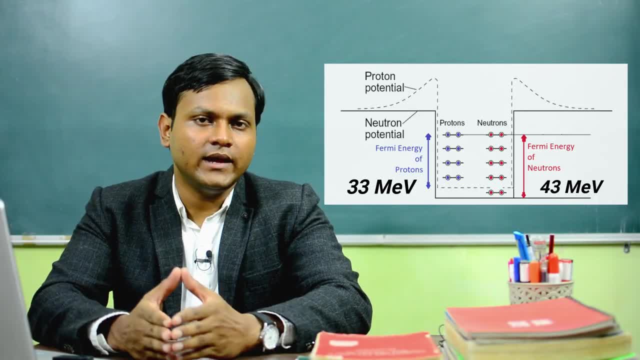 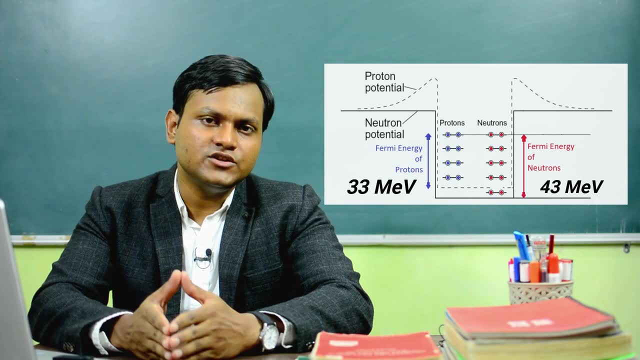 that for the case of neutrons, the Fermi energy is around 43 mega electron volts and for the case of protons, the Fermi energy is around 33 mega electron volts. Now, of course, the Fermi energy of protons and neutrons are going to be: 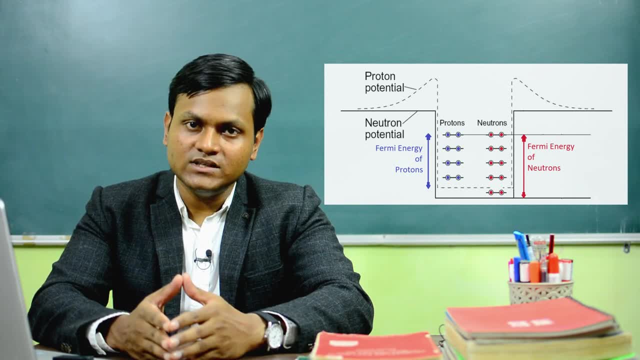 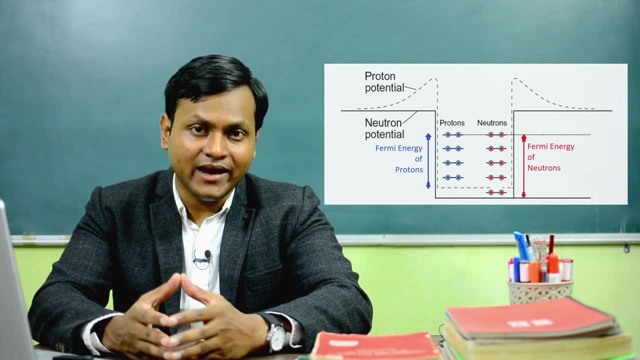 different because in a medium to large sized nucleus the number of neutrons is more than a number of protons. So if the number of neutrons are more than the neutron density is going to be higher compared to the proton density and because of this reason the Fermi energy of the neutrons is greater than the. 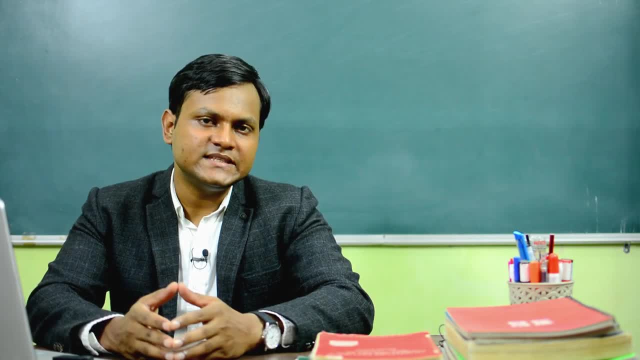 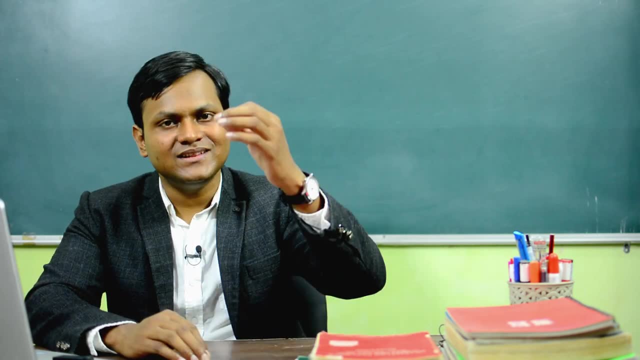 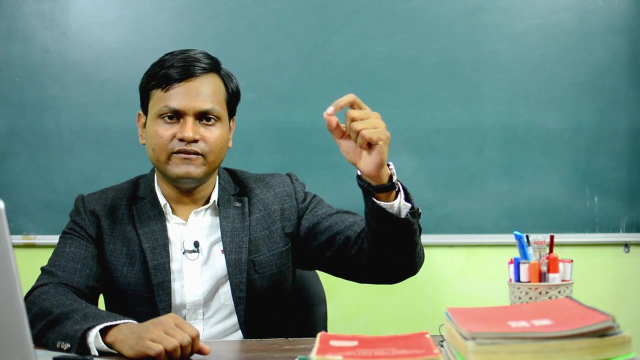 Fermi energy of protons. Now, since Fermi energy is basically the energy difference between the highest occupied state and the lowest occupied State, we can use this to calculate the, the potential depth of the nuclear potential well itself. so if you look at the case of the neutrons, the highest occupied state is at the energy level of 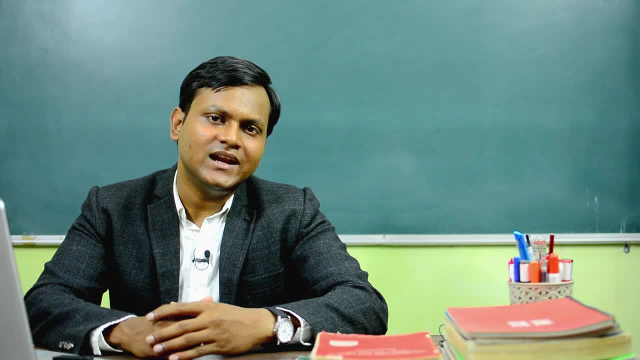 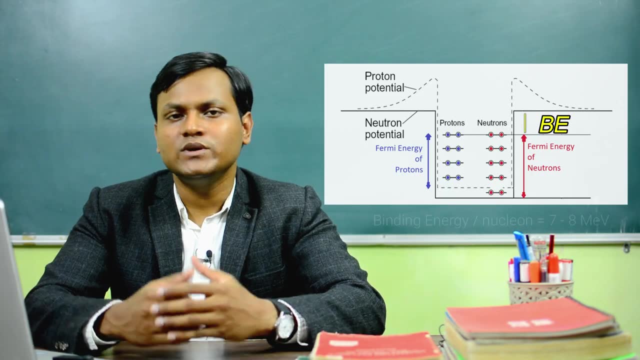 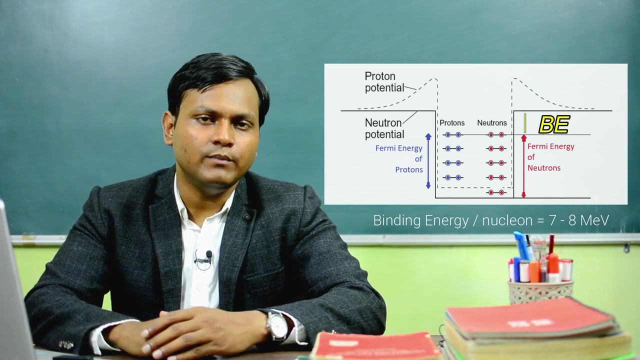 around 43 mega electron volt. what is the amount of energy that I have to give to the nucleus to free the neutron in the highest occupied state? that is known as binding energy. so what is the binding energy per nucleon? for neutron in a nucleus it is around seven to eight mega electron volts. so if seven to eight mega 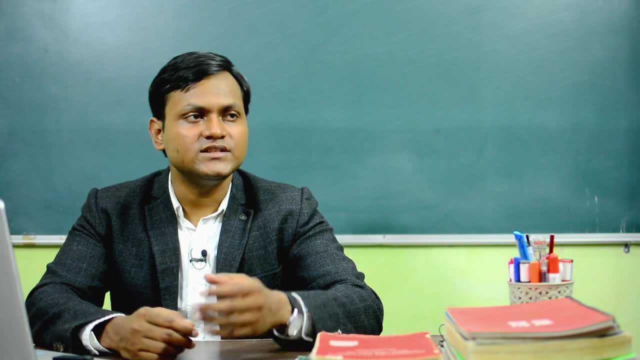 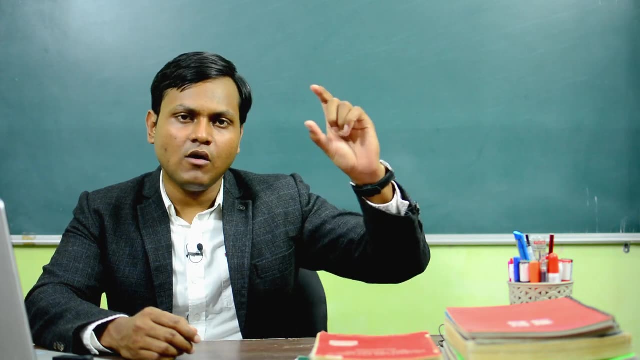 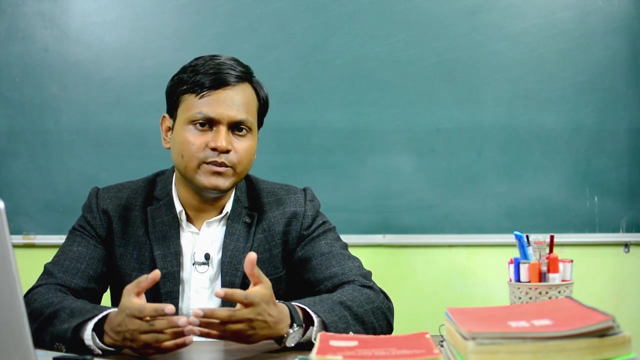 electron volts is the amount of energy that I need to provide to a nucleus to free the highest occupied neutron. then what is the potential depth? the potential depth is basically the sum of the binding energy per nucleon plus the Fermi energy, so the potential depth can therefore be approximated to be equal to. 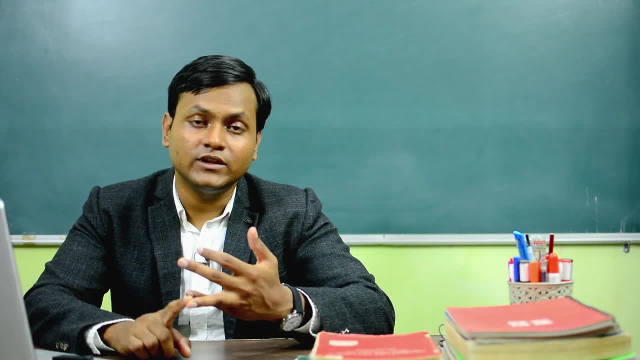 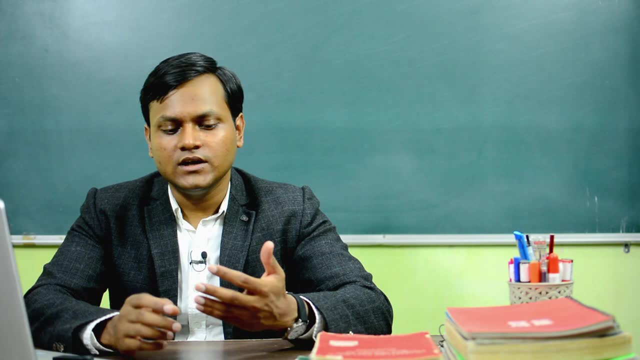 43 plus 7 mega electron volts for the case of neutrons, which adds up to around approximately 50 mega electron volts, and for the case of protons, the total potential depth is around 50 mega electron volts, and for the case of neutrons, the total potential depth is around 33 plus 7 mega electron volts. 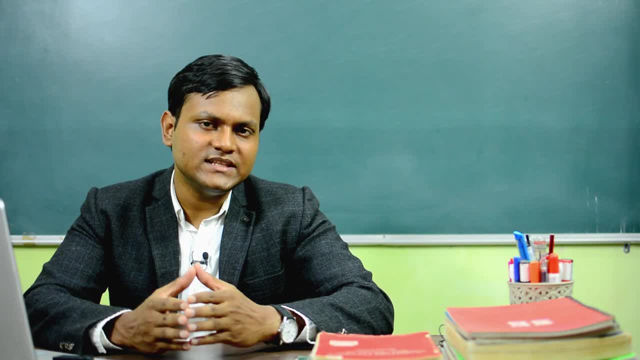 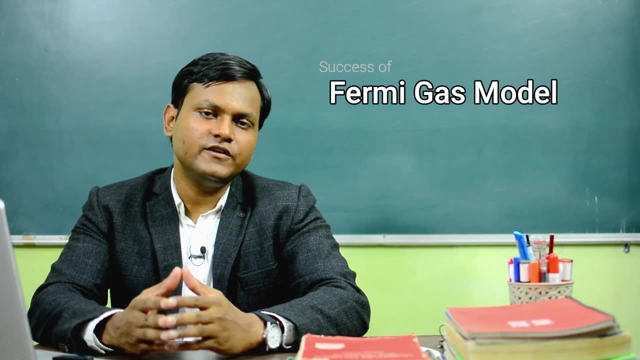 which approximates to 40 mega electron volts. so, as you can see, the potential depth of neutrons and protons is not the same, which is kind of obvious. what are some of the successes of the Fermi gas model of the nucleus? since Fermi gas? 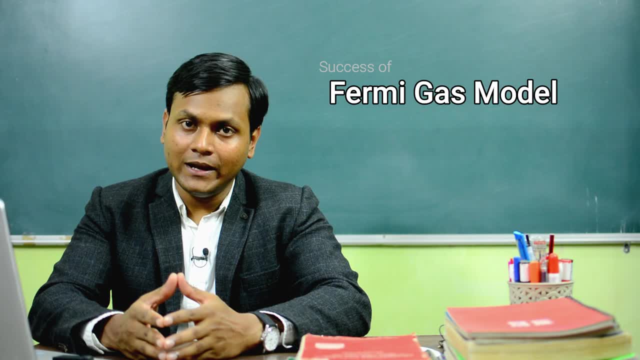 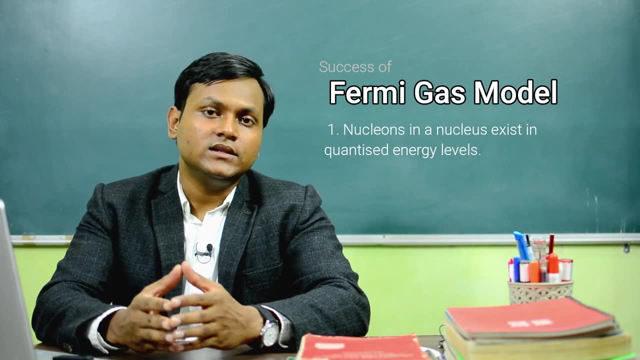 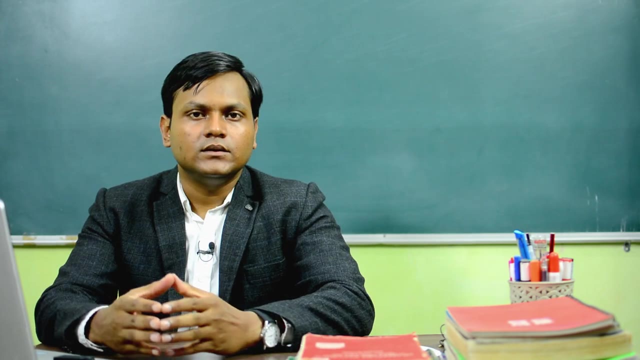 model assumes that the particles are bound in a potential. well then, these particles will only exist in discrete or quantized energy levels, so that that means the nucleon particles, both neutrons and protons, have their distinct energy level diagram inside the nucleus. the second is that it 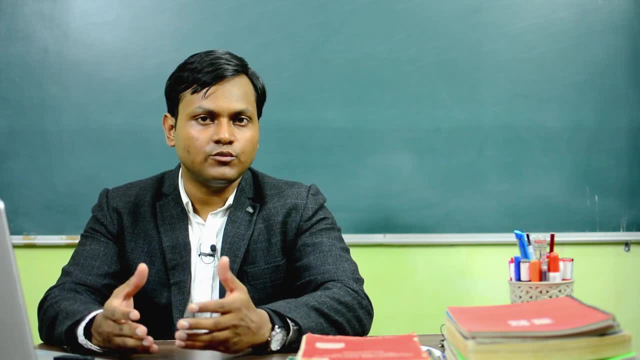 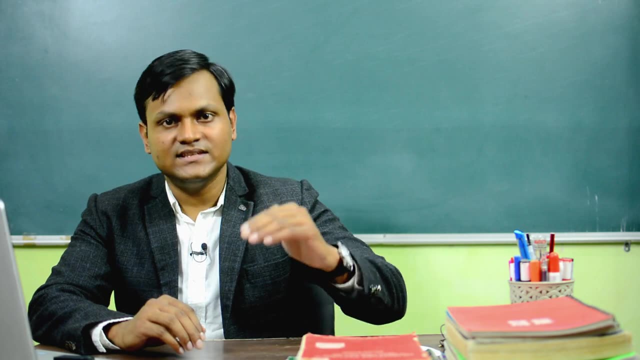 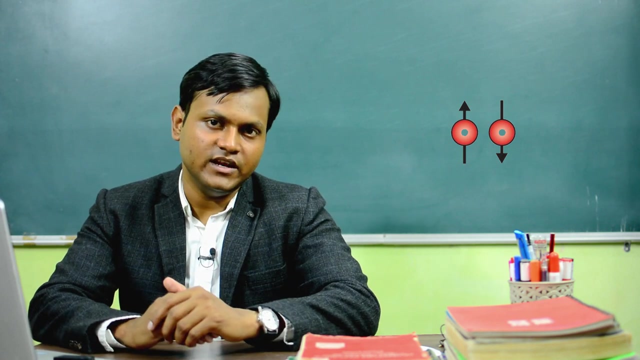 explains the pairing of neutrons and protons. so since neutrons and protons are fermions and they occupy this distinct quantized energy levels, then no more than two of these particles can exist in one given energy level. so you have two neutrons of opposite spin pairing up to fill one given energy levels and two protons of opposite spin pairing up to fill its own energy levels. this is the reason why even-even nuclei are much more stable compared to even odd nuclei, and which are much more stable compared to odd-odd nuclei. so even-even nuclei are those nuclei we have which have even number of protons and even number of. 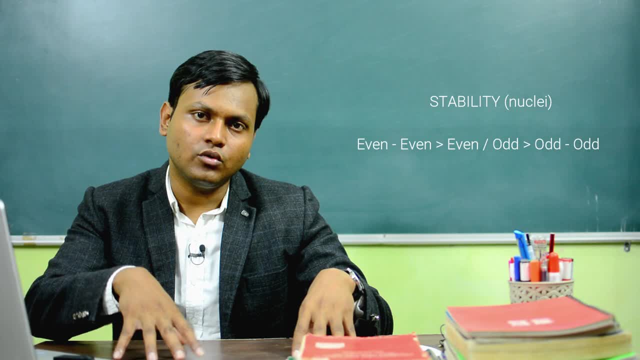 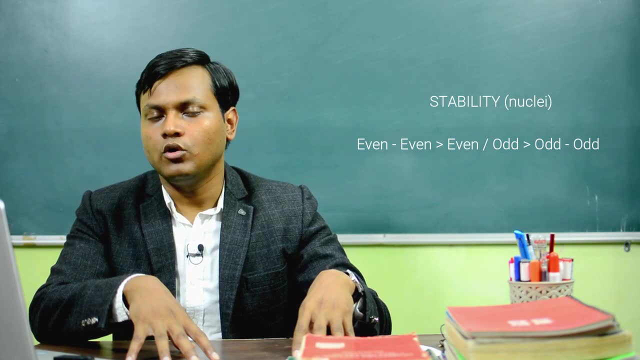 neutrons. so what happens if a nuclear configuration of even number of protons and even number of neutrons, it leads to complete filling up of the energy levels? there is no unpaired neutron or proton. because of this, this kind of a configuration is much more stable compared to an even odd nuclei or an odd 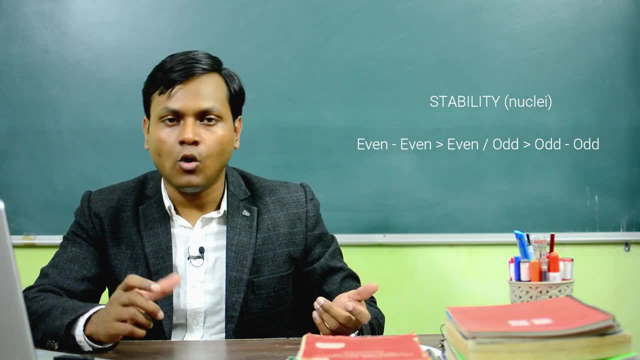 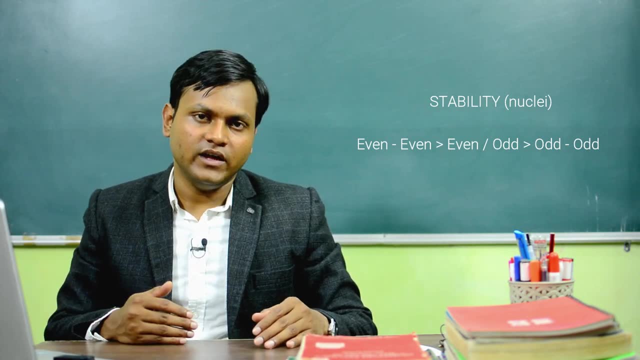 nuclei which basically consists of an even number of protons and an odd number of neutrons, and vice versa. In this case you have an unpaired neutron or a proton and the least stable are those configurations which have odd, odd nuclear configuration, which have odd number of neutrons. 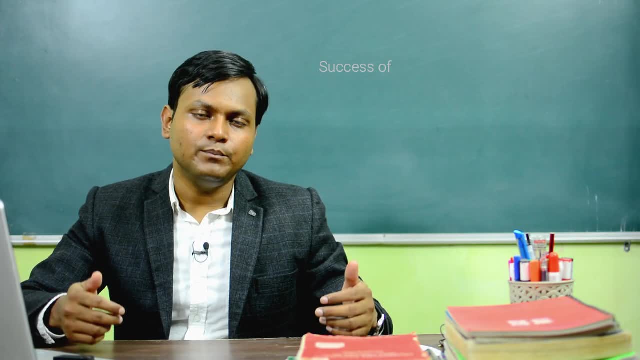 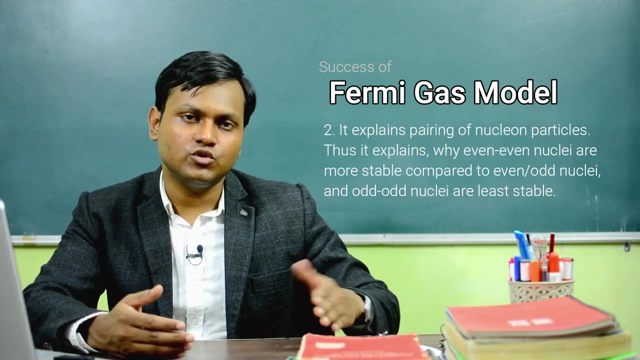 and odd number of protons basically means that you have two unpaired neutron and proton respectively. So in a way this explains why even even nuclear structures are much more stable, because it leads to pairing of neutrons and protons which fill up the energy levels of a nuclear. 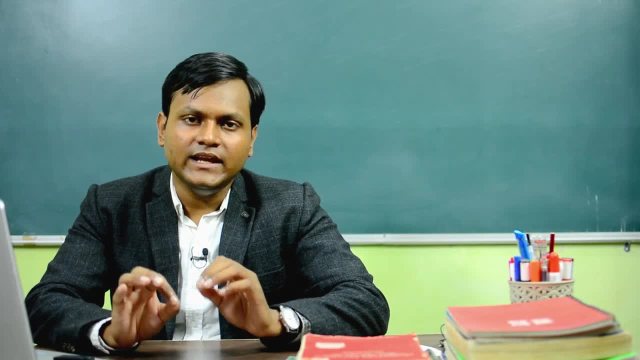 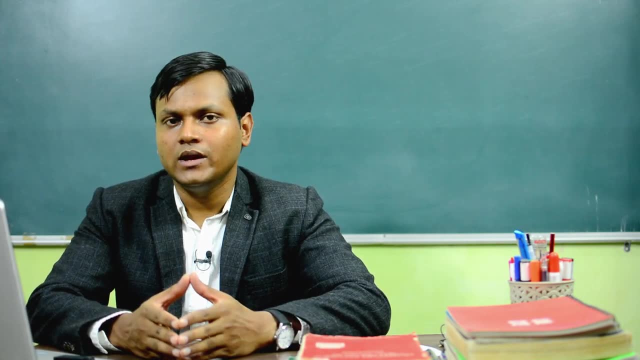 energy diagram. And lastly, but most importantly, it also gives an explanation for the beta decay processes. Now, the number of neutrons and protons in medium to large nuclei are not necessarily equal, but they rather follow what is known as the NZ graph or the stability curve of 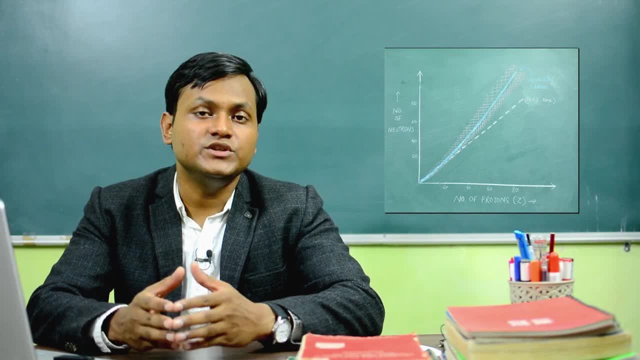 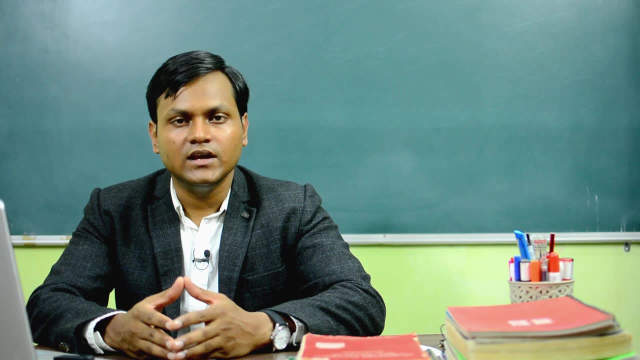 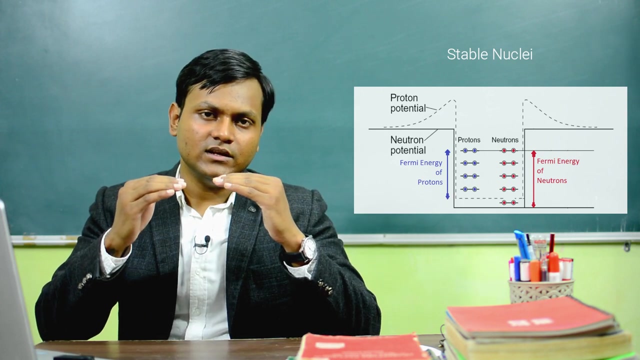 an NZ graph, Those nuclear configurations which deviate from the NZ graph usually undergo beta decay process. So why there's these beta decay processes? So if you look at the energy level diagram of any given nucleus, then the Fermi energy for a stable energy level diagram is usually the same for both neutrons and protons.